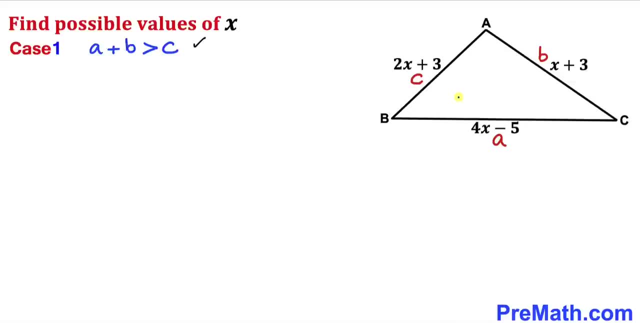 A plus B is greater than C. Let's go ahead and fill in the blanks. In our case, A is 4x minus 5 and B is x plus 3.. Let's add them up: 4x minus 5 plus x plus 3 is greater than our. C is 2x plus. 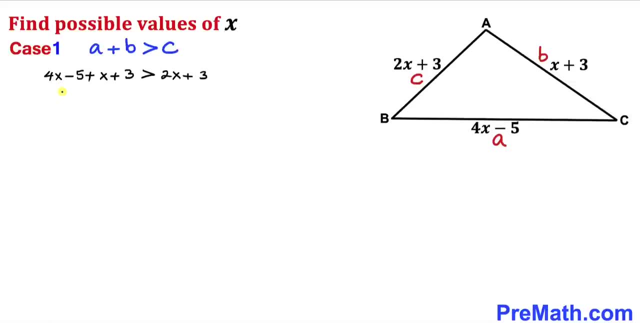 3. Let's go ahead and combine the like terms on left hand side, so we got: 5x minus 2 is greater than 2x plus 3. now let's go ahead and subtract 2x from both sides, so this is gone. so we ended up with: 3x minus 2 is greater than 3. let's go here. 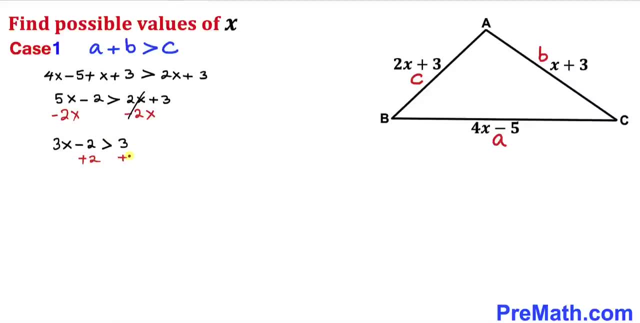 and add 2 on both sides, so this is gone as well. so we got 3x is greater than 5 and finally, let's go ahead and divide both sides by 3, so therefore we are going to have x is going to be greater than. 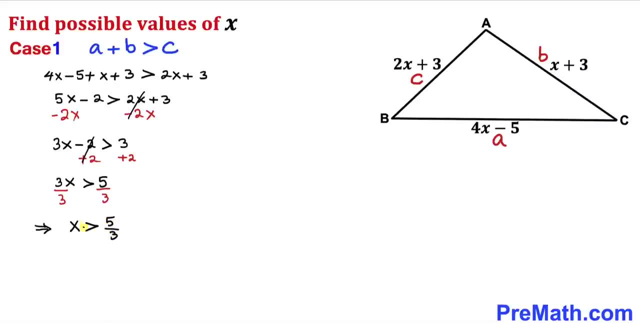 5 over 3, this inequality. so thus, for our case 1, we ended up with our this inequality: x is greater than 5 over 3, and here's our next step. let's go ahead and discuss our case 2, when a plus c is greater than b. now let's go. 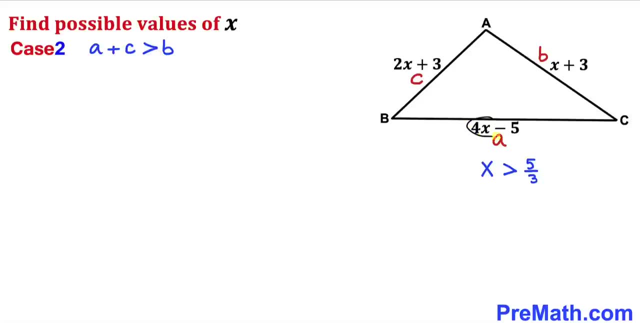 ahead and fill in the blanks. in our case, a is 4x minus 5 and c is 2x plus 3. let's go ahead and add them up. so 4x minus 5 plus c is 2x plus 3 is greater than b. in our case is x plus 3. now let's go ahead and. 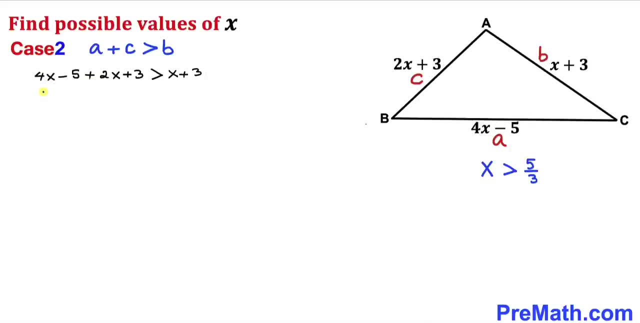 combine the like terms on the left hand side, 4x plus 2x, is going to give us 6x minus 2 is greater than x plus 3. for our case, x is greater than 2, so now let's go ahead and have x at the time that we add 5 x minus. 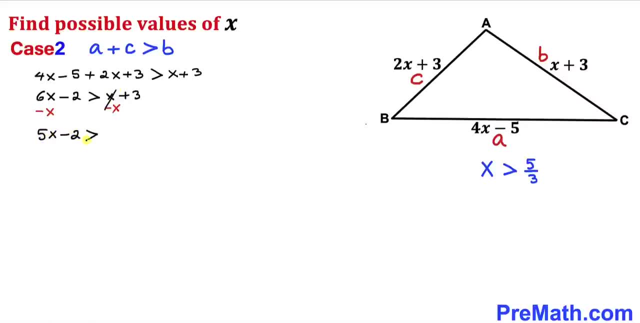 2 on both x plus 2 is equal to 5, and you can see, c is greater than 3, less than 6 x 1 is equal to 2, and so here we arestorm by both sides. now let's go ahead and subtract 1x from both sides. this is gone, so we. 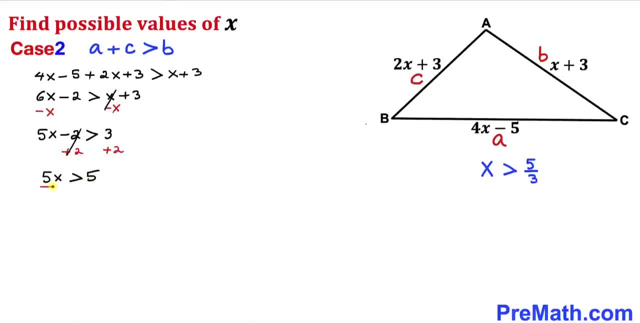 ended up with 5. five, let's divide both sides by five. so therefore, our x value turns out to be greater than one, and this is our another inequality. so thus, for our case two, our value for x turns out to be: x is greater than one. and finally, we got this case three, when b plus c is greater than a. let's go. 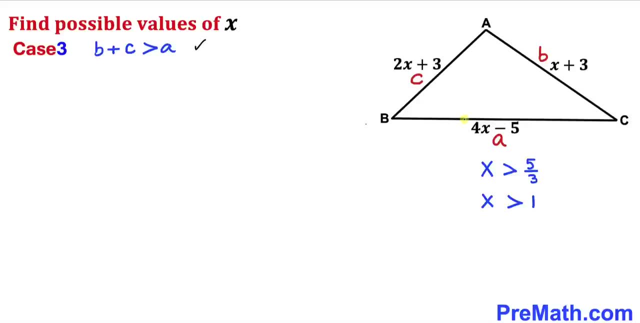 ahead and add these: one in our case b, is x plus three and c is two x plus three. let's go ahead and add them up: x plus three plus two. x plus three is greater than a. in our case is four x minus five. let's go ahead and combine the like terms on the left hand side. 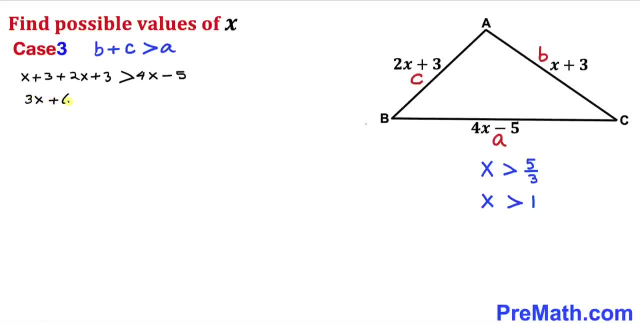 we got three. x plus six is greater than four. x minus five. let's go ahead and subtract three x from both sides. we can say: this is gone, so six is greater than x minus five. let's go ahead and add five on both sides, so this is gone. so we ended up with 11. 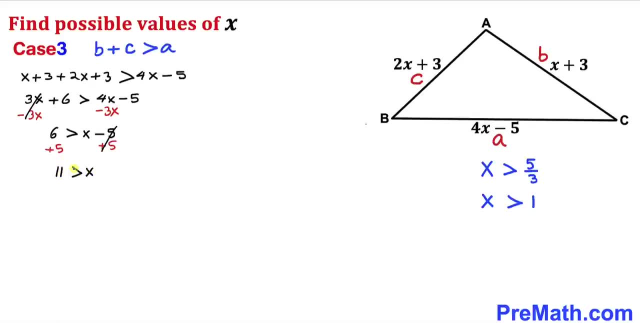 is greater than x, and if we can write it the other way around, so x is going to be less than 11.. it doesn't make any difference whatsoever writing this way. so this is our before and after, and this is our third, and this is our third and last and now let's go ahead and